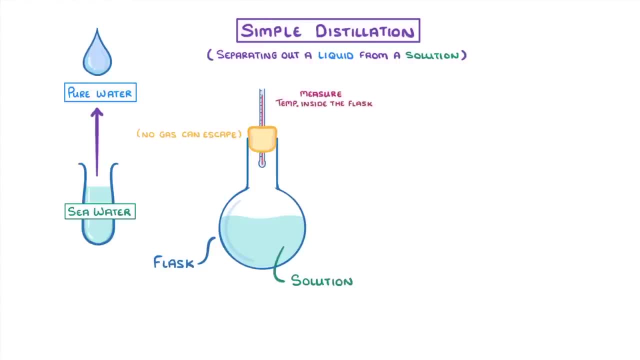 the bung so that we can measure the temperature inside the flask. Next, we have our condenser, which consists of a main pipe surrounded by a water jacket which contains a stream of continually flowing cold water, with the water being fed into the. 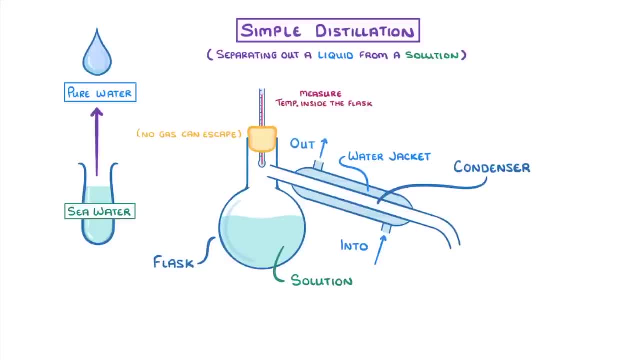 water jacket at the bottom and coming out at the top. Then, beneath the end of our condenser we'll have some sort of beaker to capture our pure liquid. And finally, we're going to need some sort of heating device like a Bunsen burner, which we place under the flask. 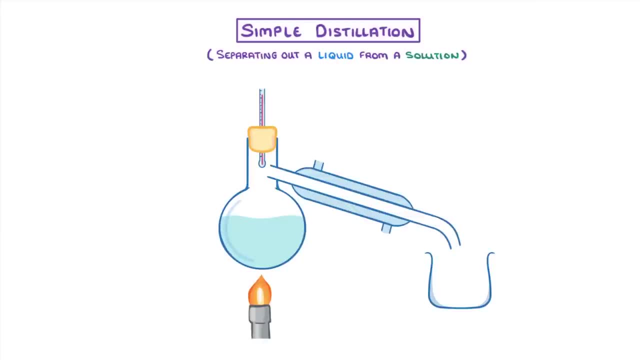 Our first step is to heat up the mixture so that the liquid that we want evaporates. As it rises to the top of the flask, the pressure will force it down the condenser and, because we're pumping cold water through the water jacket, the vapor will cool and 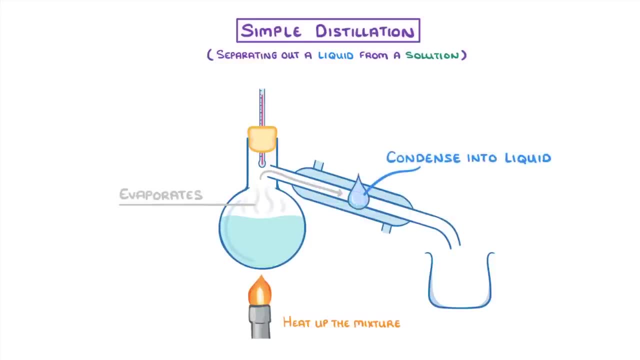 condense into liquid form, which will then run down the pipe and collect in the beaker. So in our case, as we heat the seawater, we'll get more and more pure distilled water, and it'll eventually all we have left in the flask is salt. 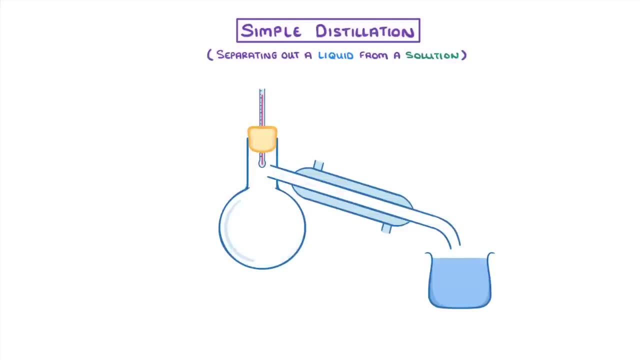 Now imagine instead that we were trying this technique with a different mixture, one containing some different liquids like methanol, ethanol and troponol. We'll need a sorta of a bunch of oxygenwart liquid which, invisible to your eye, will. 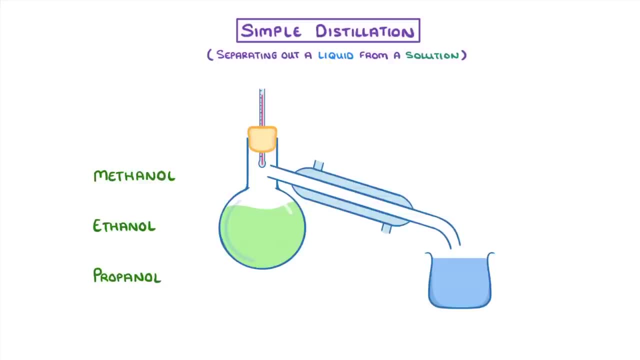 allow us to get some oxygen, what we're faring from, Because these liquids all have similar boiling points. when we heat them, more than one of them will evaporate, and so they wont be separated out into pure substances. In this case, we'd have to use a different technique called fractional distillation. 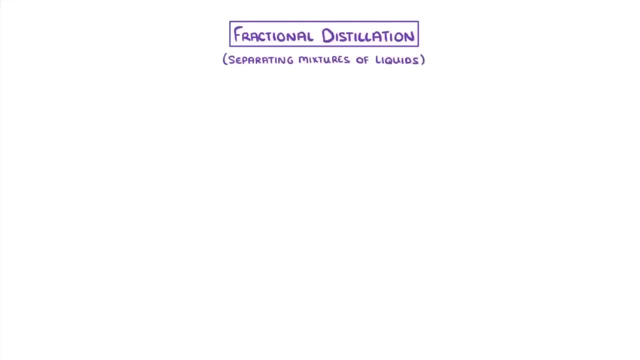 which is the main technique used for separating mixtures of liquids as they rotate. The equipment for this is pretty similar, But instead of the gas part that causes it to evaporate, we'll need some a derivative of this liquid. But instead of this location of the alcohol we'll need some a miniaturized liquid. and now there's not any peaks at all, so all that gas and bog will remain in the liquid. 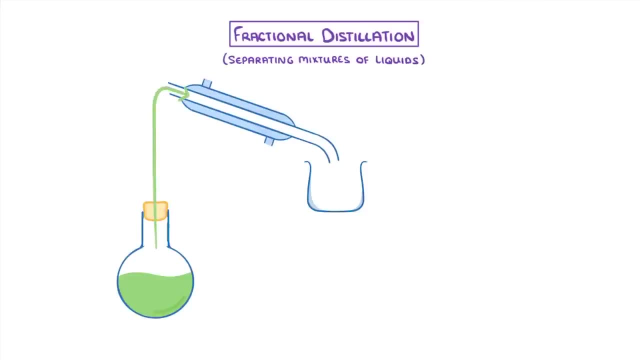 we'll need some a miniaturized liquid passing straight from the flask into the condenser. the vapours have to first pass through a fractionating column which has two key features. One is that it's full of little glass rods which 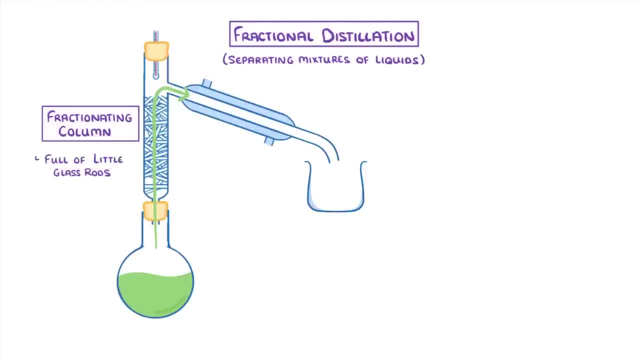 provide a really high surface area, And the other is that, because the column is so tall, it's actually cooler at the top than it is at the bottom. To understand why this is important, let's imagine that we were trying to separate those three liquids that we mentioned before- Methanol, ethanol and propanol, which all have similar 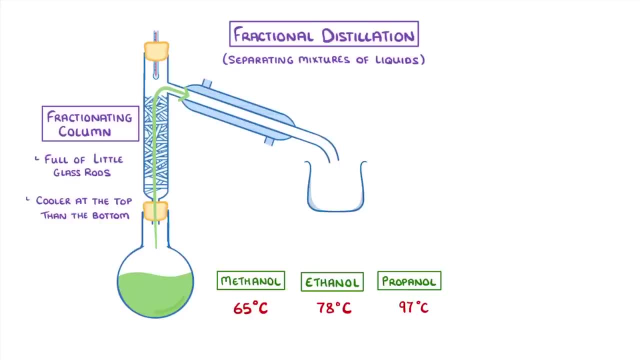 boiling points, although you don't need to remember them. And before we continue, just be aware that in real life these would all be colourless, not green. We're just showing them as green to make it easier to follow along. Now, because methanol has the lowest boiling point, we'd heat the mixture to around 65. 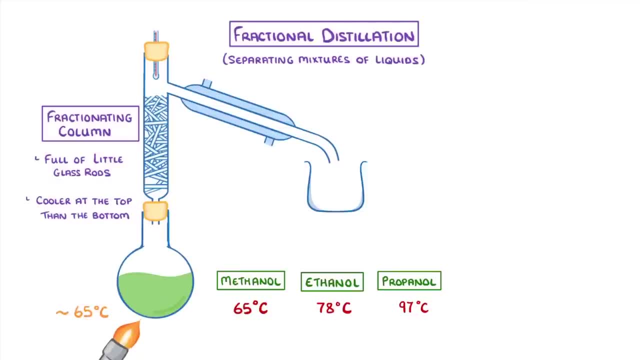 degrees. first, This would cause the methanol to evaporate and then rise up the fractionating column. It would then pass into the condenser and condense into liquid methanol, which we would then collect in our beaker. However, just by chance, some of the ethanol, and maybe 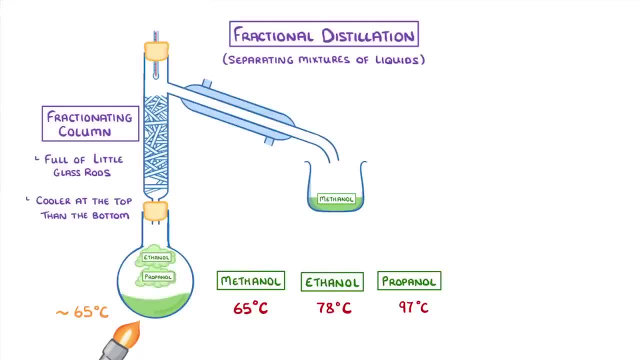 even propanol would also evaporate, But as they rise up the fractionating column and come into contact with all of those glass rods which are much cooler than their boiling point, they'd condense back into liquid form and fall back into the flask. This means that the only liquid that will get out the other 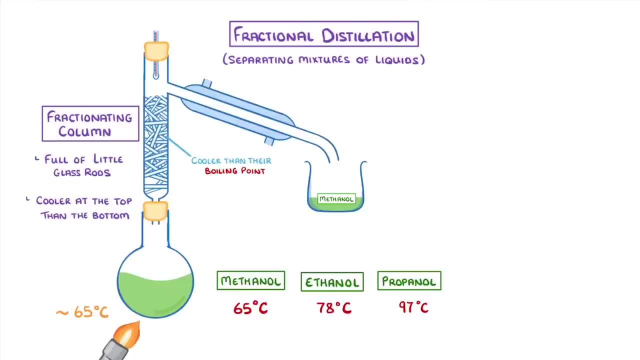 side will be pure methanol. The next step would be to do the same thing all over again for ethanol, by raising the temperature to around 78 degrees Celsius. At this point, all that should be left is the propanol, So we could just assume that. 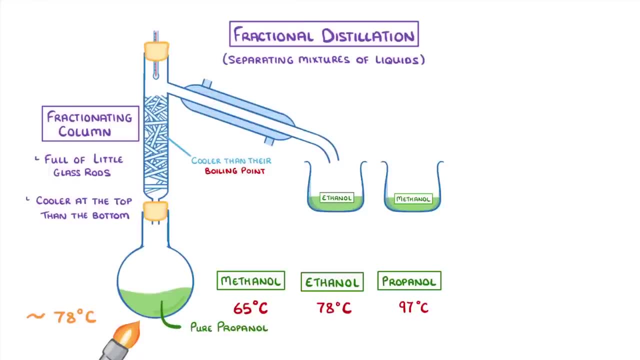 what we have in the flask is pure propanol, or we could raise the temperature again to boil off the propanol, just to make sure. Anyway, that's all for today, So hope you enjoyed this video and I'll see you in the. next one.